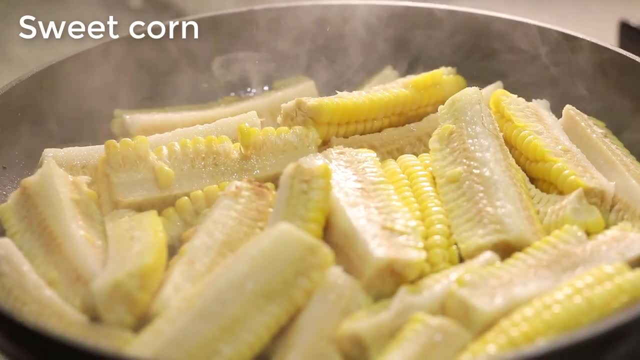 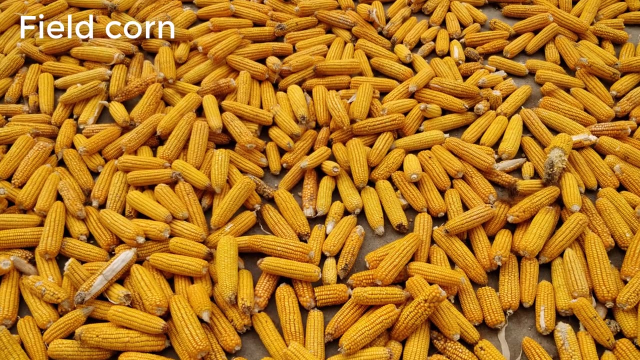 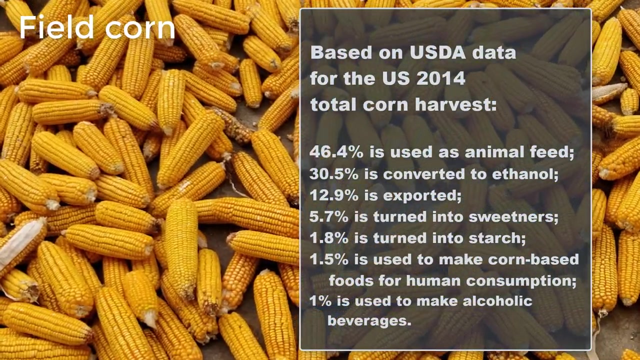 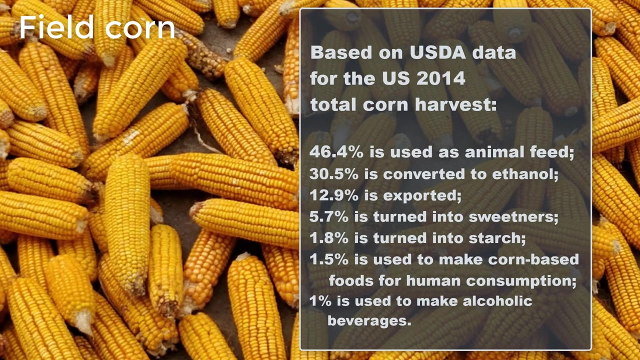 it is soft, creamy and sweet, ready to be eaten raw or slightly cooked. Filled corn is usually harvested when the kernels are fully mature and dry. It is used to make a variety of products, including animal feed or corn-based food products for people, such as cornmeal, popcorn, corn oil, corn syrup, ethanol and alcohol. 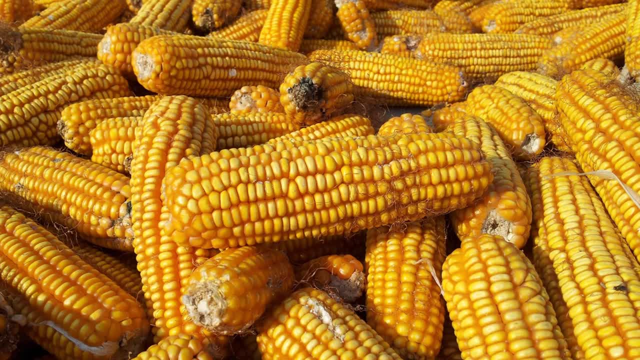 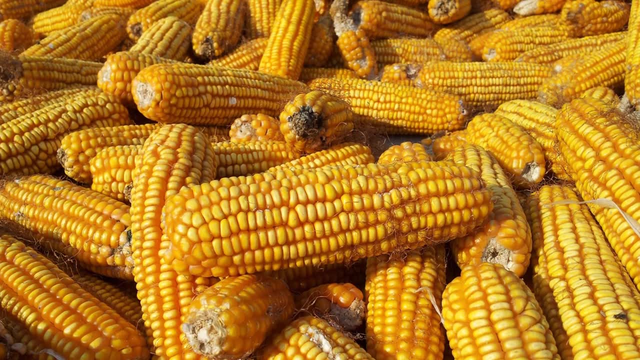 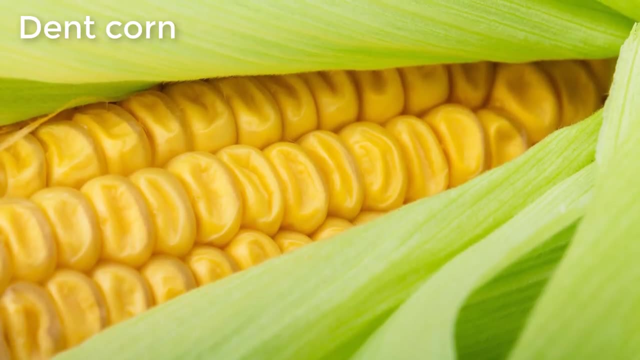 Filled corn further consists of the following types of varieties: Most filled corn grown in the United States today is dand corn, also known as grain corn. It received its name because of the small indentation or dand at the crown of each kernel on a ripe ear of corn. 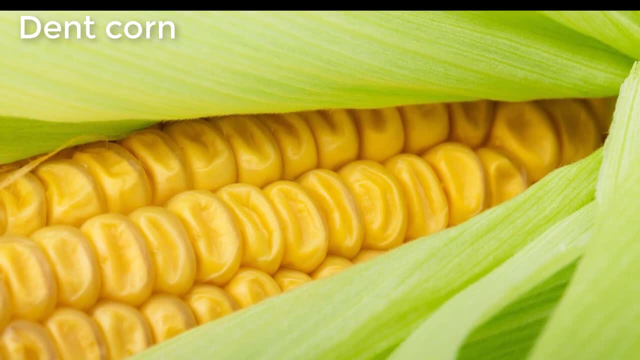 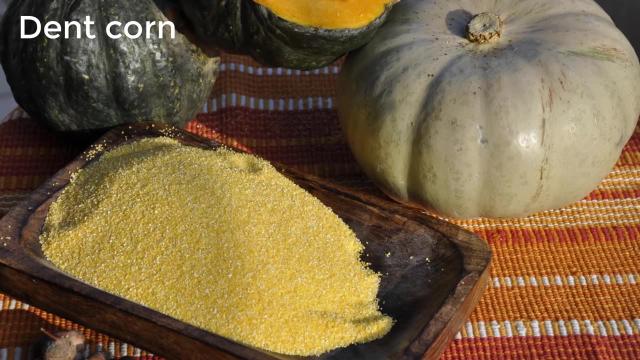 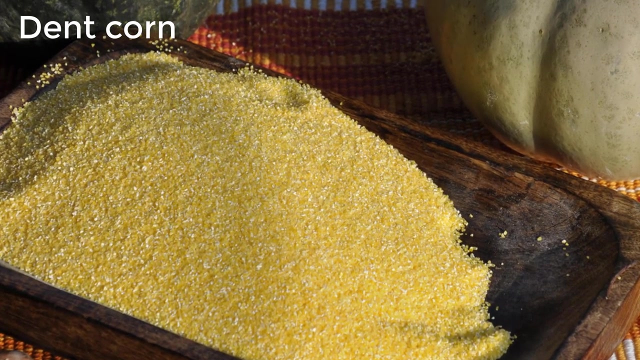 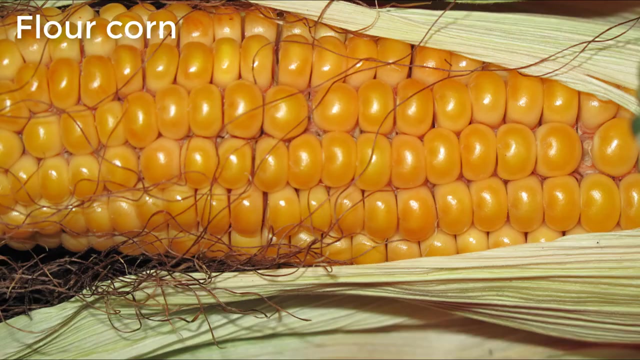 Dand corn is used as animal feed and in manufacturing such foods as cornmeal, corn chips and tortillas. Starch derived from this high starch content variety is turned into plastics, as well as fructose or corn syrup, which is used as a sweetener in many processed foods and soft drinks. 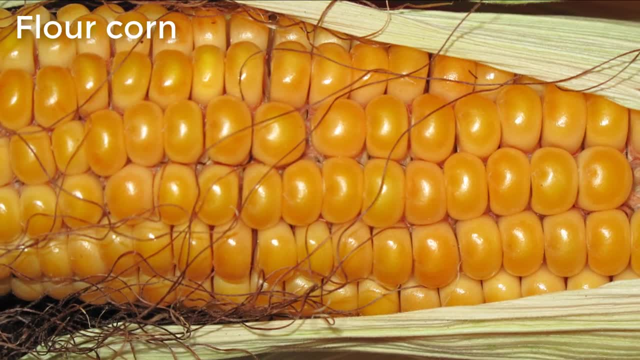 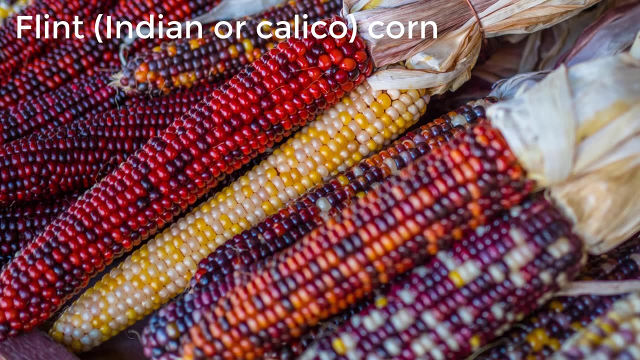 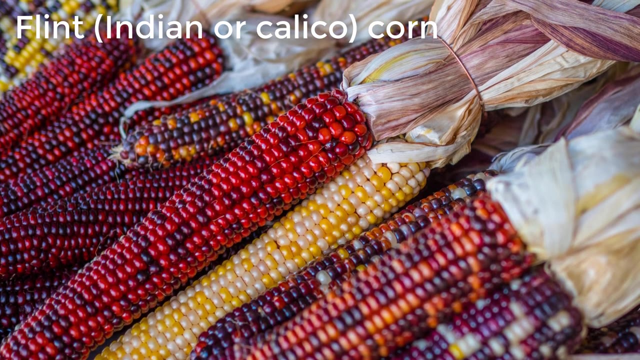 Flour corn is composed largely of soft starch and easy to grind into flour. Flint corn, also known as Indian or calico corn, is a group of the oldest varieties of corn grown mainly by indigenous communities of Central and South America, as well as the Southwestern US. 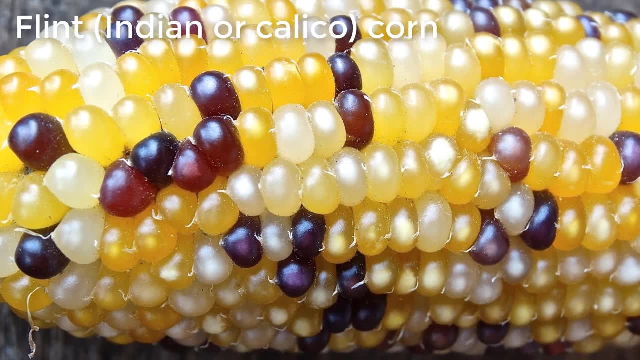 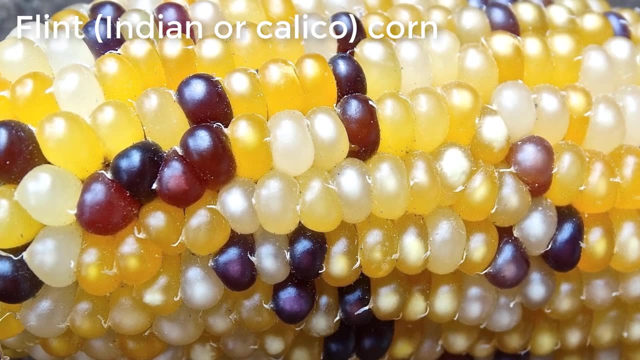 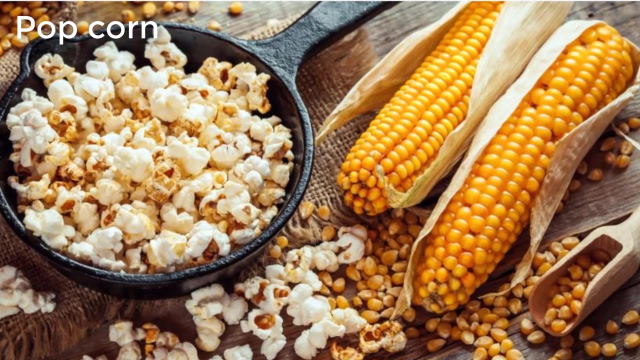 It comes in many colors, such as blue, purple, pink and red. Its kernels are harder than dand corn, yet flint corn, if prepared correctly, has higher nutritional value than any other types of corn. Popcorn is the oldest type of domesticated corn. 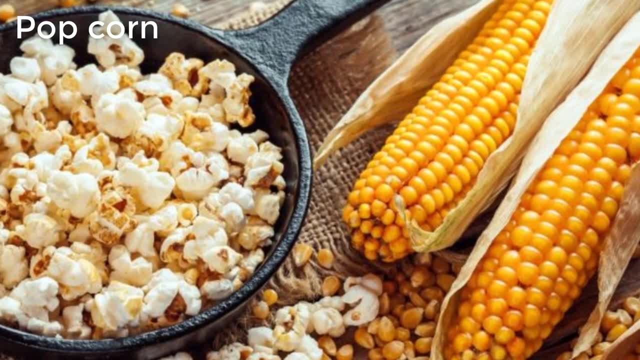 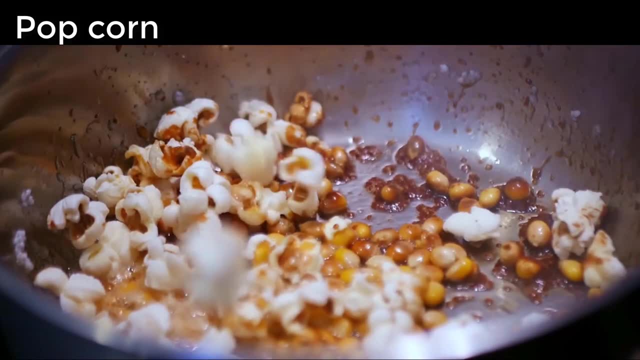 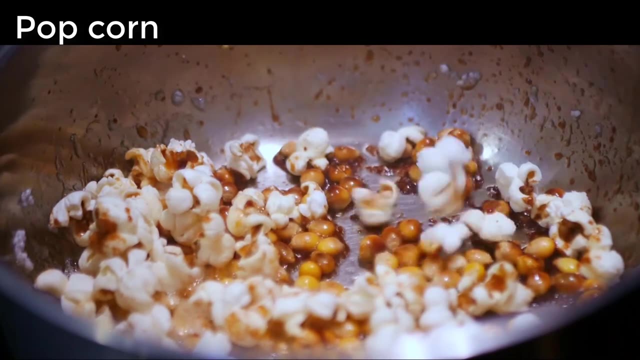 It is very similar to flint corn and has a hard, moisture-sealed hull and a dense, starchy interior that puffs when heated. Most of the world's popcorn is grown in the United States: Corn Belt of Illinois, Indiana, Iowa, Kentucky, Michigan, Missouri, Nebraska and Ohio. 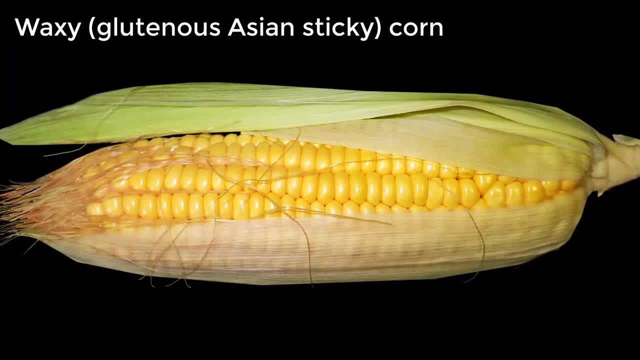 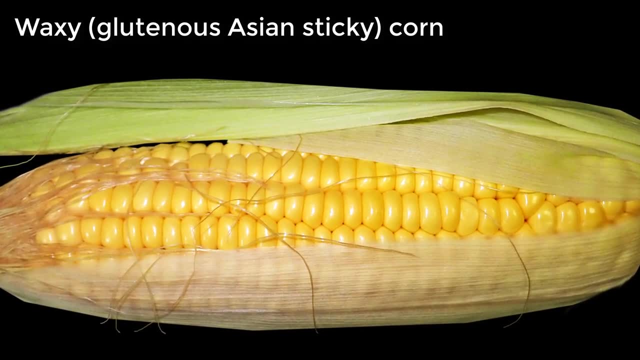 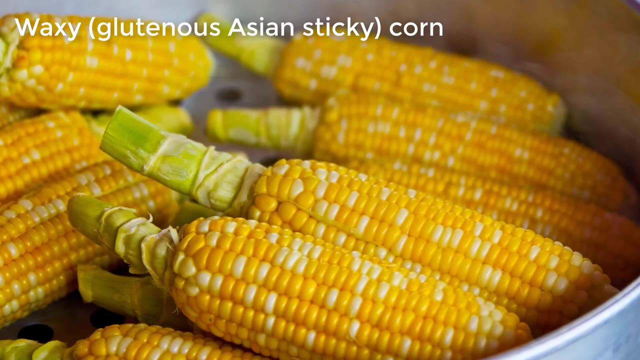 Wax and gluten. The uniqueness of sticky corn originates in Southeast Asia and is characterized by its sticky texture when cooked, as a result of larger amounts of amylopectin, a component of starch. My Vietnamese neighbors grow this kind of corn in their garden and I ate it with them on numerous occasions. 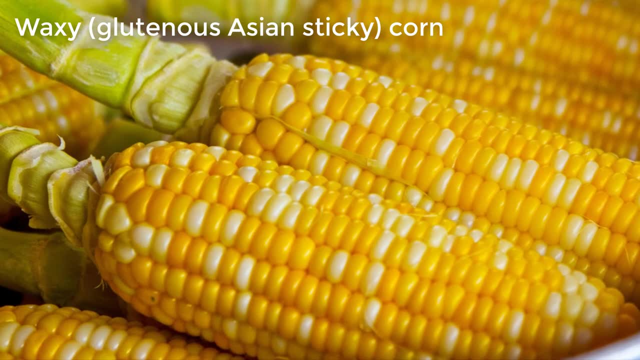 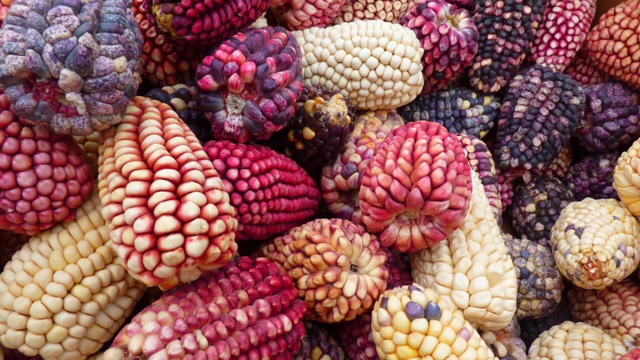 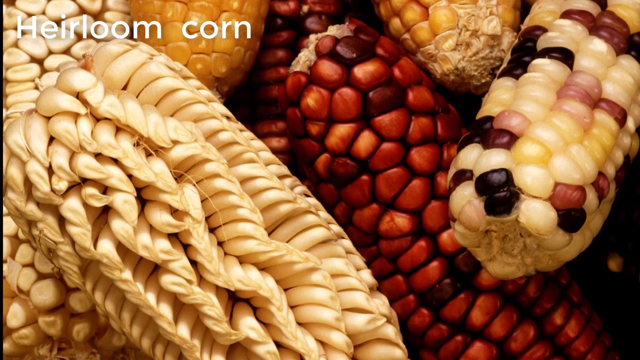 It is as good as sweet corn with a slightly more dense and sticky texture. There is also a number of heirloom varieties that are not grown widely yet have their own niches here and there. One of such types is called pod corn, for example. 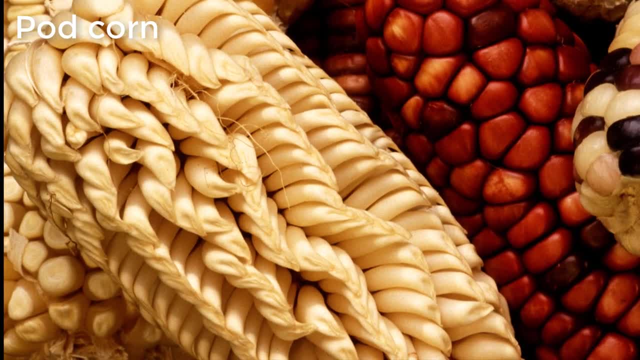 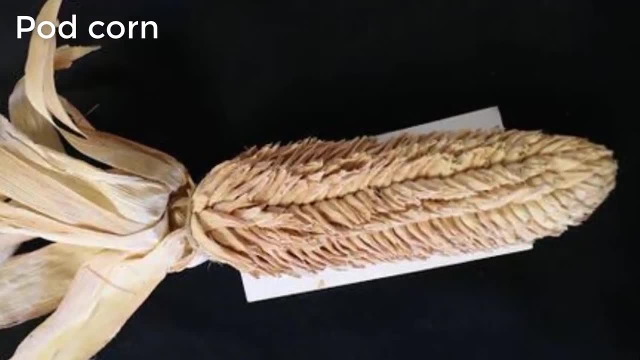 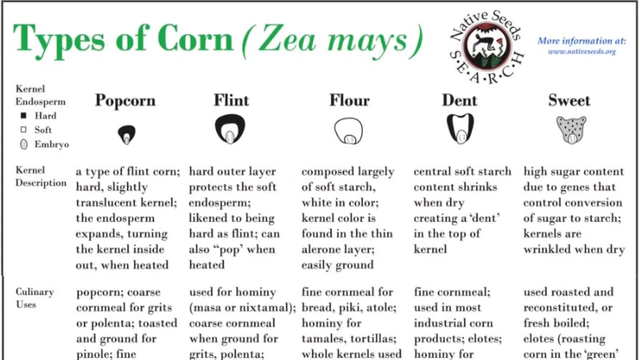 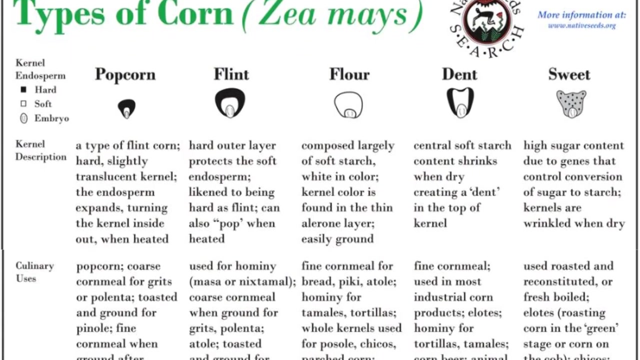 It has each of its kernels enclosed in husks, as well as the whole ear, like in the other types of corn. All types of corn cross-pollinate easily. Not all varieties fit neatly into one specific type of corn. There are many varieties that combine characteristics of two or more types of corn. 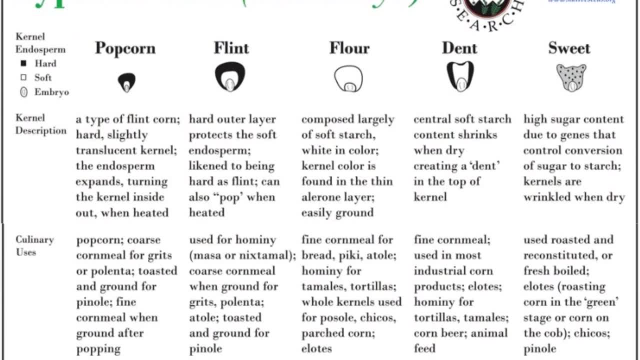 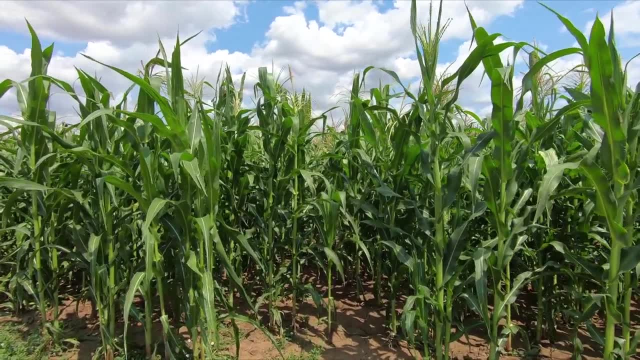 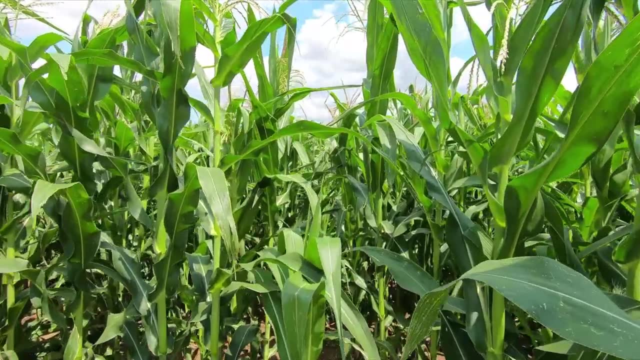 For example, both flint and flower corn characteristics can be present in the same variety. If you want to grow several varieties, you have to plant them at a distance of at least 250 feet between each other. Corn is pollinated by wind, so that's another factor to consider. 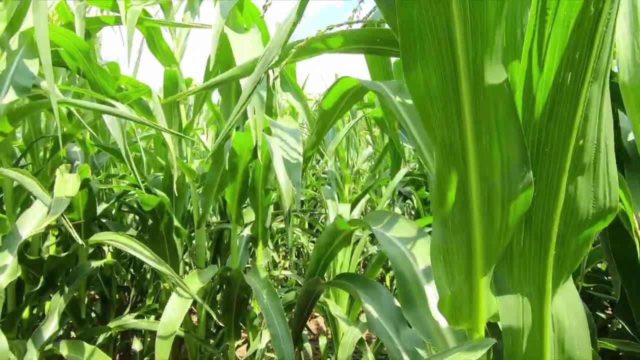 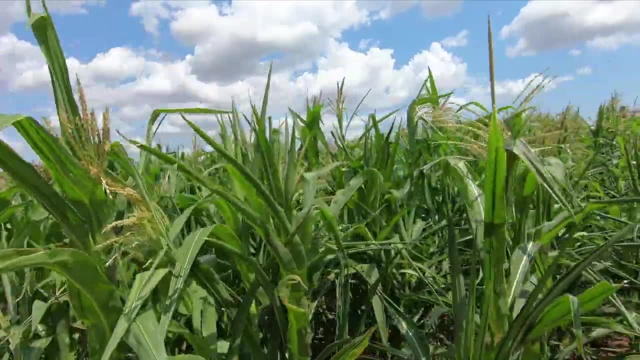 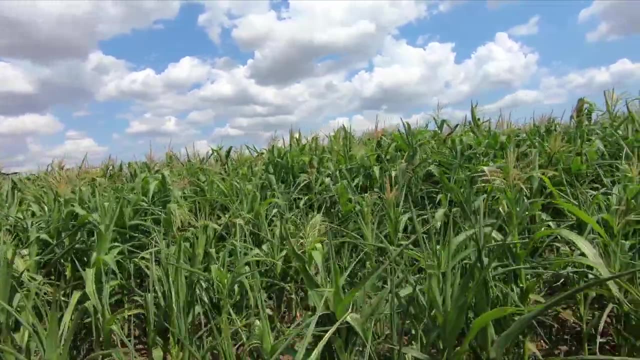 Higher winds mean longer distances between the varieties. Different varieties could be also planted at different times so that they do not bloom at the same time, Or you choose varieties that mature at different times. It is recommended that there is a two-week period between the tussling. 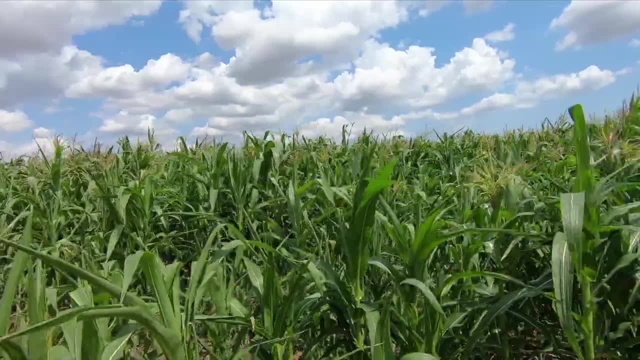 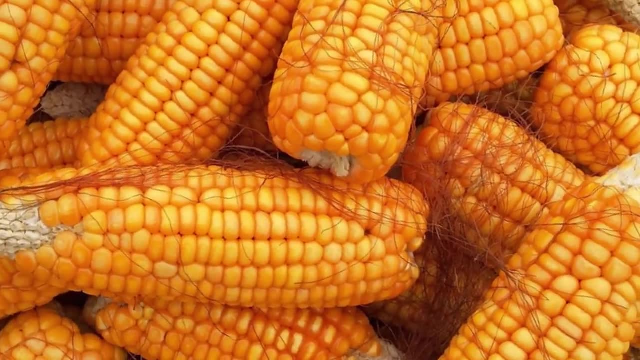 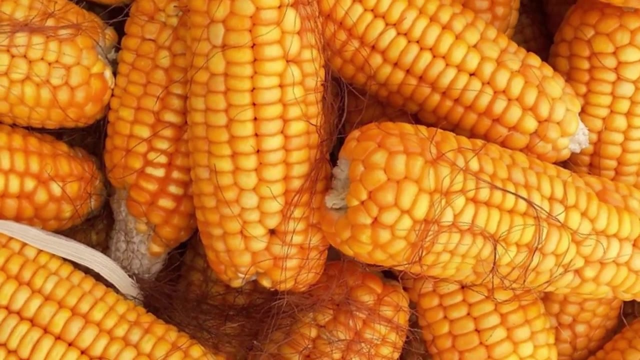 or flowering of the male flowers of the varieties grown close to each other to prevent cross-pollination. In the next video we are going to look at the nutrition that corn brings to our table, at the pros and cons of having it as part of our diets. 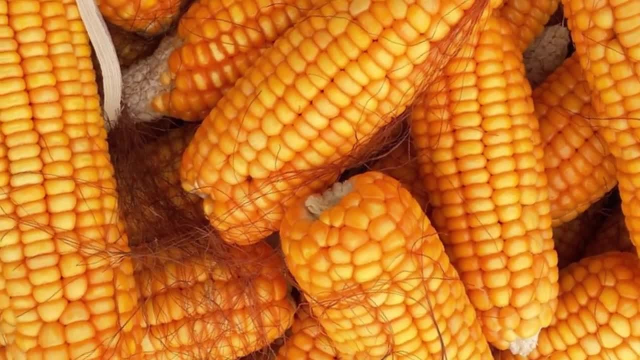 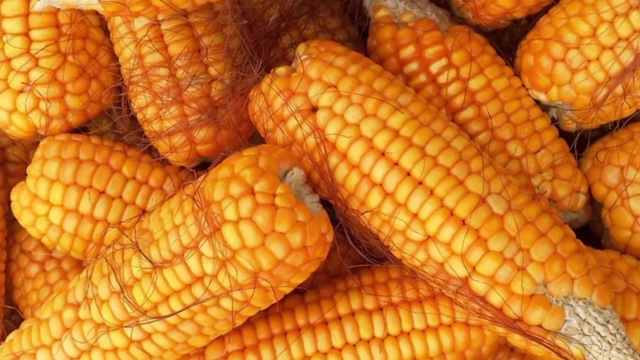 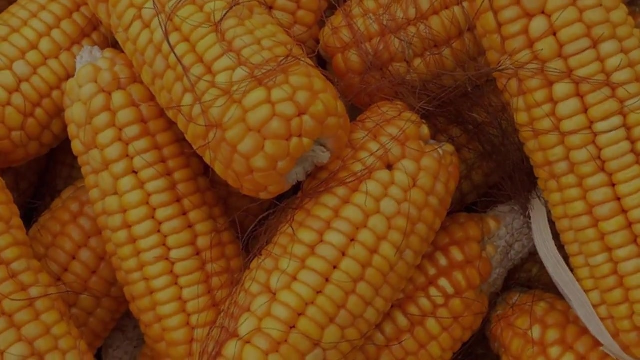 If you want to learn about the botany and origins of corn, go to the Part 1 of this series. Thank you for watching.